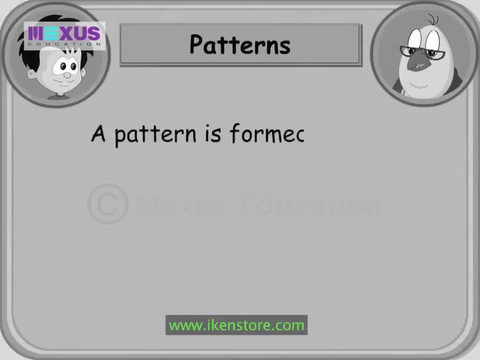 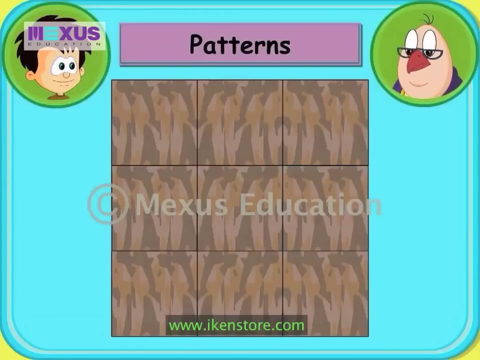 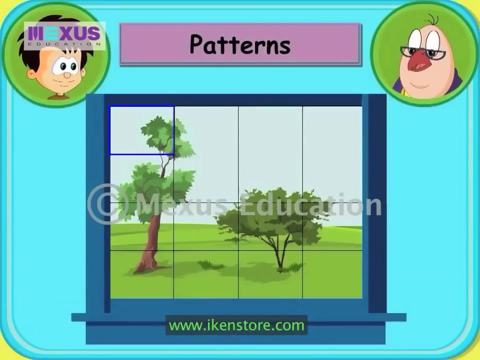 A pattern is formed when a set of shapes, numbers or designs are repeated. Patterns are repeated over and over again. Patterns are found everywhere in our world. You can see patterns in the floor tiles of your room, in flowers, in architecture and in objects that we use every day. 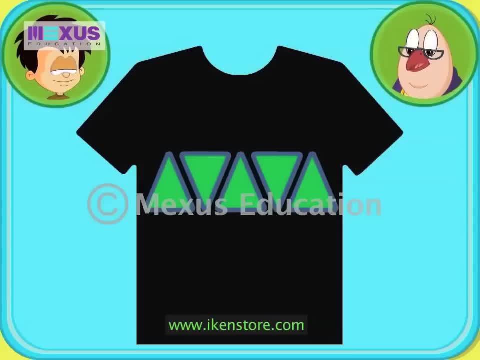 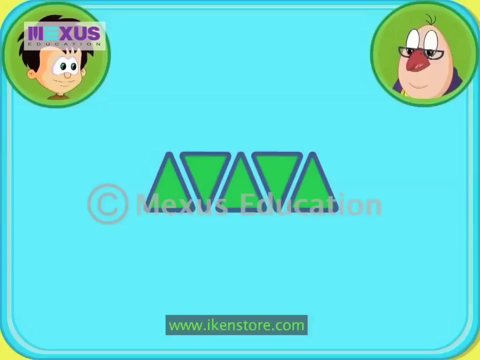 Take a look at this t-shirt, JC. The triangles on it form a pattern. The pattern is formed by a triangle, followed by an upside-down triangle being repeated over and over again. Once you identify a pattern, you can take it forward yourself. 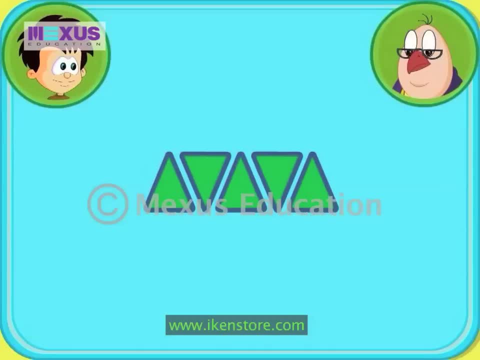 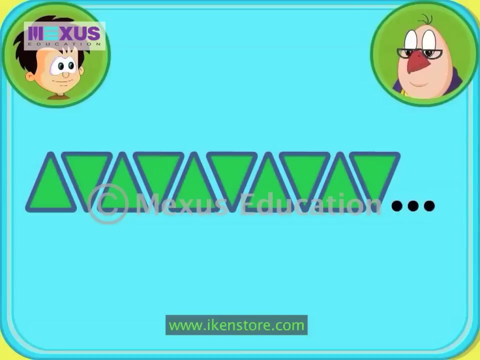 Completing patterns is quite easy. Yes, JC. All you need to do is first decide the shapes or numbers that you will use and arrange them in a particular pattern. Let's take a look at some patterns and see if we can complete them ourselves. 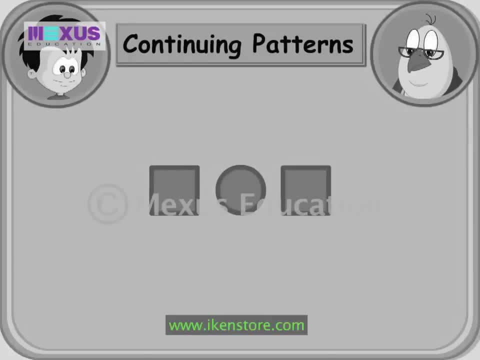 Let's look at this pattern now. You must have noticed that in this figure a circle follows a square and a square follows a circle. This is the pattern rule of this figure. Patterns which show this type of continuity are known as continuing patterns. 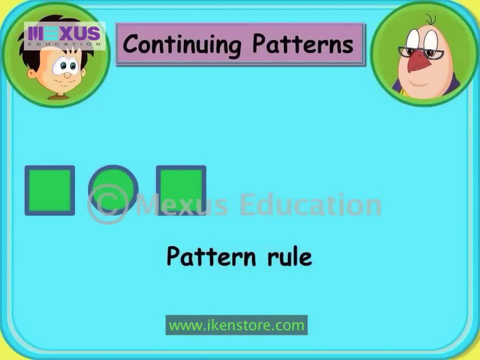 Let's complete this pattern. To complete this pattern, we will continue the series of a circle followed by a square, And a square follows a circle. This is the pattern rule of this figure. Now look carefully. Can you identify the pattern rule here? 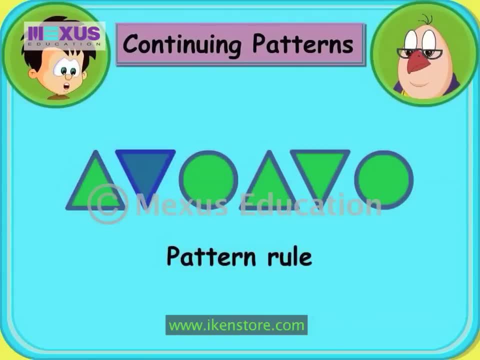 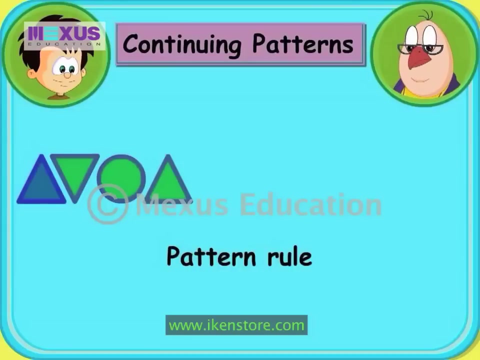 Yes, Dr O. A triangle is followed by an upside-down triangle and then a circle. These three shapes are repeated once more in the pattern. Now let's repeat these shapes and continue the pattern. Do you know, JC, that even numbers follow patterns? 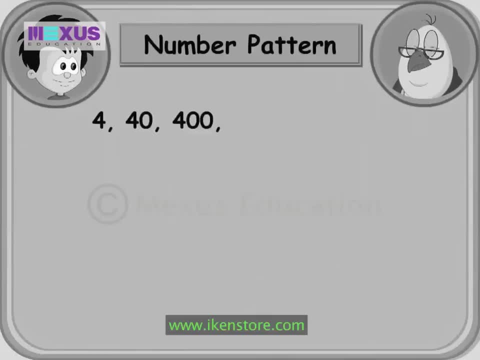 Let me show you an example. Can you identify the pattern rule here? 4, 40,, 400, 4000,? um, not really. If you look closely, you will see that even numbers follow patterns. If you look carefully, you will see that a previous number, when multiplied by 10, gives the next number. 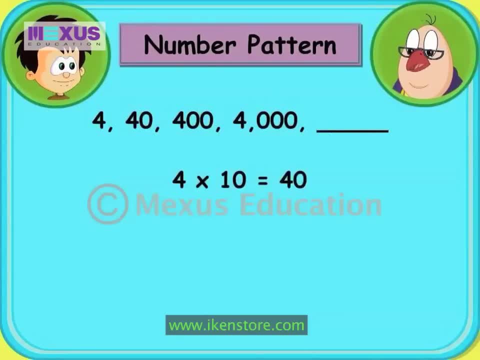 4 multiplied by 10 is equal to 40.. 40 multiplied by 10 is equal to 400.. 400 multiplied by 10 is equal to 4000.. JC, can you guess what's the next number? The next number is 4000 multiplied by 10.. 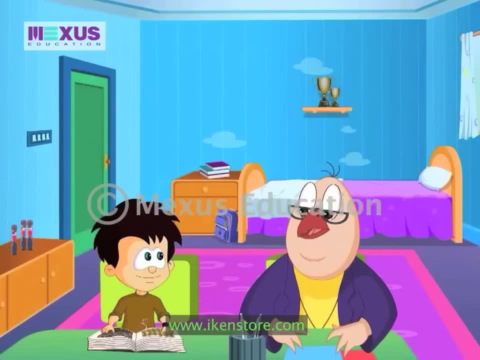 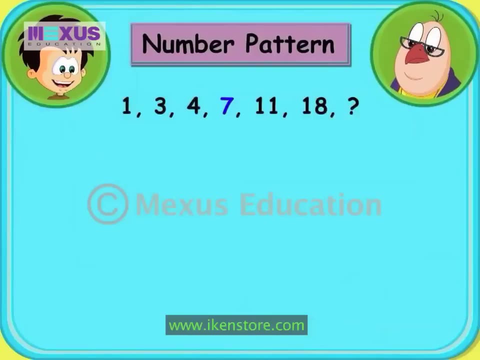 That is 40,000.. That's good. Now let's try another pattern: 1, 3, 4, 7,, 11, 18.. Now this looks tricky. Here's how We add the previous number to the current number to get the next number. 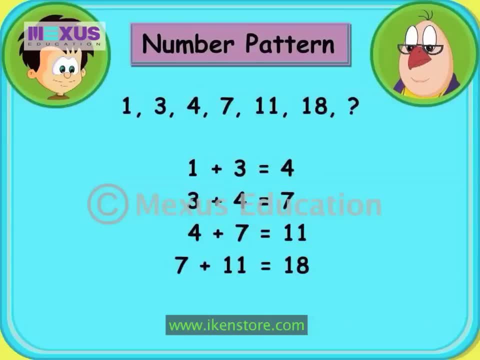 So what's the next number after 18?? The next number is 11 plus 18.. So what's the next number after 18? The next number is 11 plus 18.. So you can add: 11 plus 18 equals to 29.. 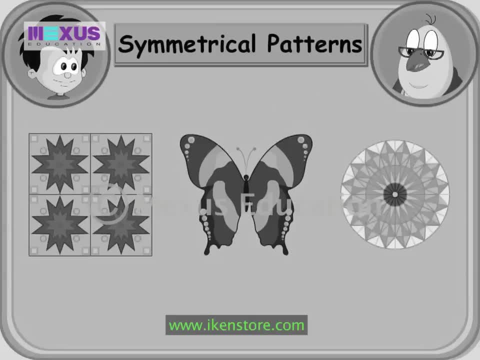 Some patterns around us are known to be symmetrical. Do you remember what line symmetry is? If a figure or pattern can be folded into mirror halves So that one half fits exactly on top of the other, then we say it has got line symmetry. 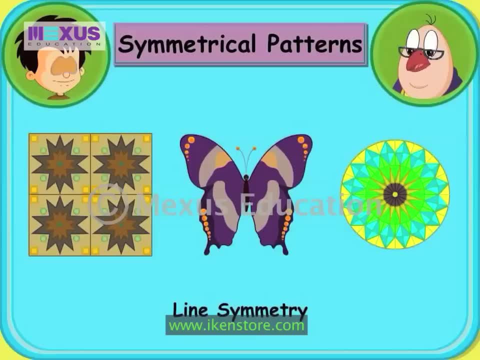 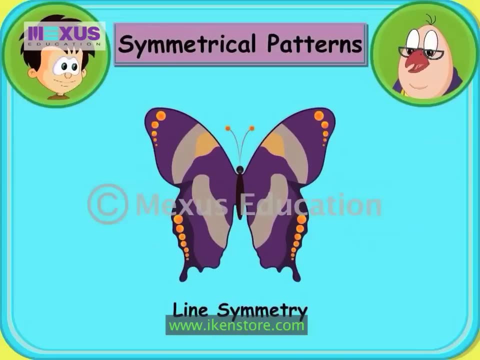 This line that divides the figure into mirror halves is called the line of symmetry. Let's take this butterfly, for example. The line of symmetry divides the figure of the butterfly into equal and identical halves. Let's complete this pattern along its line of symmetry.